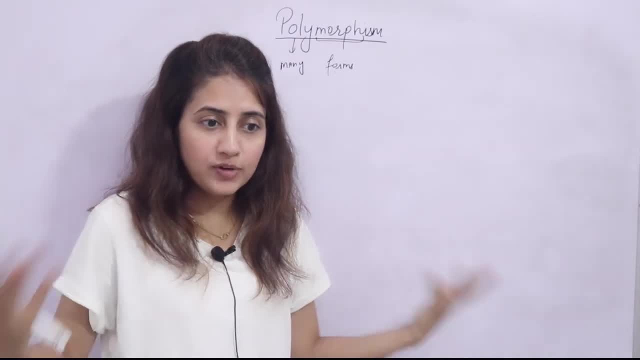 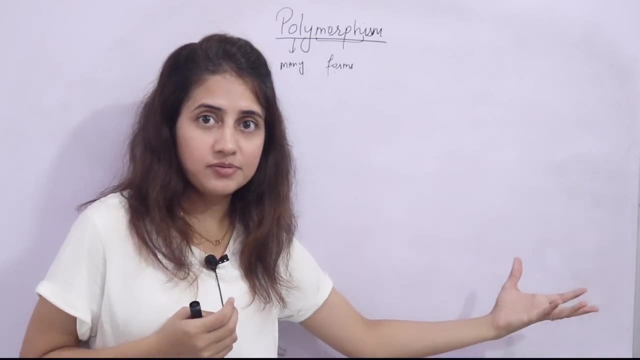 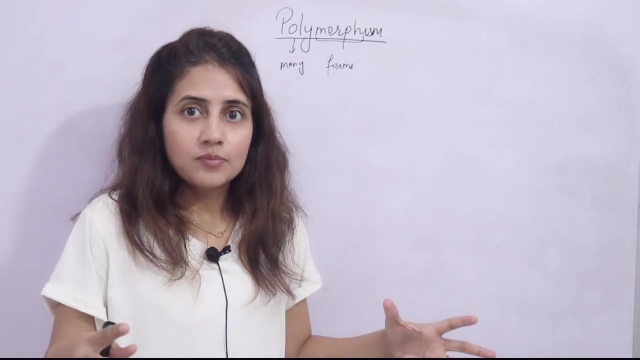 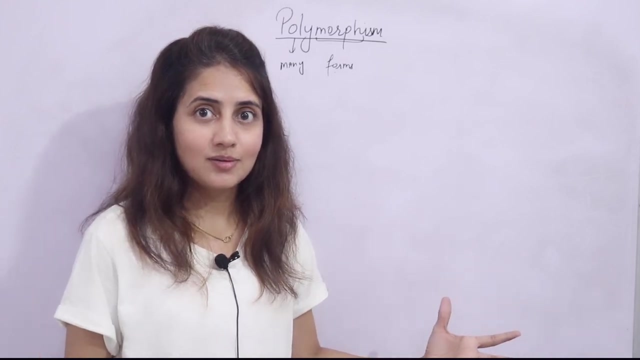 But according to the situation, I behave differently. My behavior is going to change. In front of my students, I'm something. I'm a different person With my family. I'm a different person With my friend, maybe I'm a different person. I behave differently, Right So where I am, what the situation is, what the conditions are, according to that, I changes my behavior. Right So same, like I am having multiple forms, Same. you can relate this. 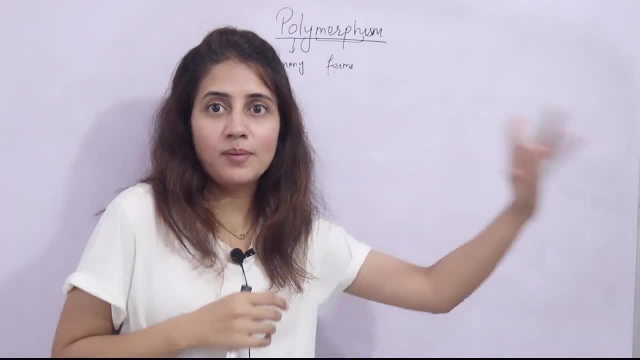 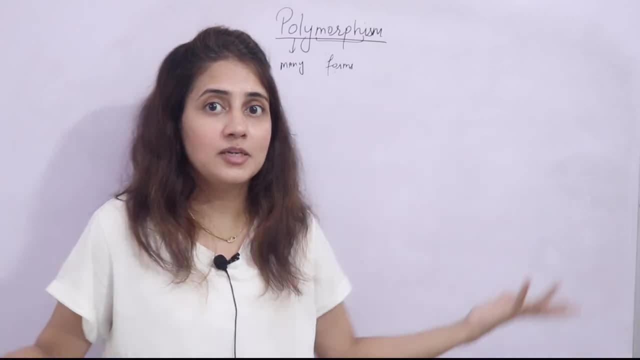 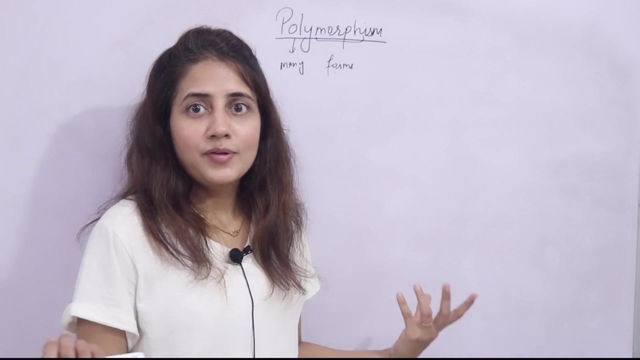 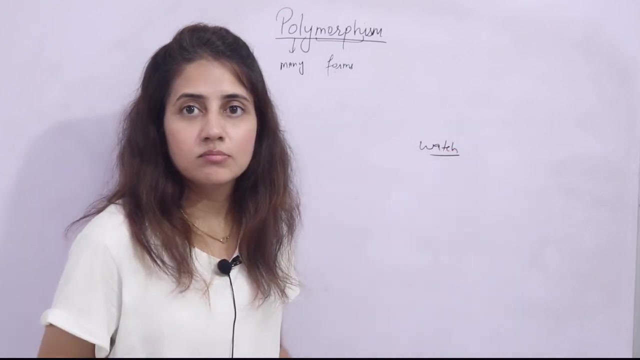 With you also. Maybe you with your friends are different. You with your family are different. You in office, if you're working, then you are different. You in college, as a student, are different. So you are also having multiple forms, Right, Many forms. So this is nothing but polymorphism. We are polymorphic Or we can say simple. some words in English like watch, Simply watch means that Rest watch also Right Watch means like: 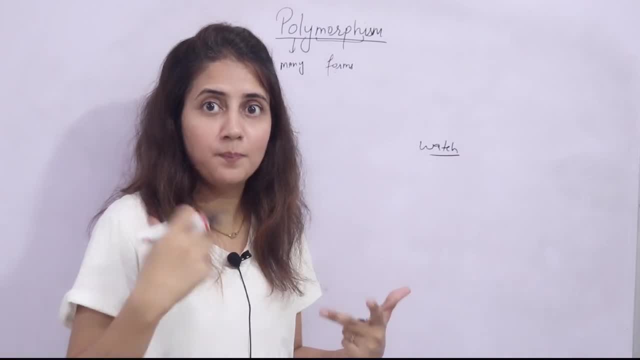 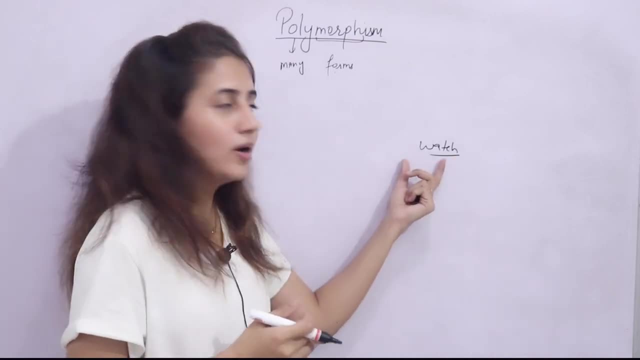 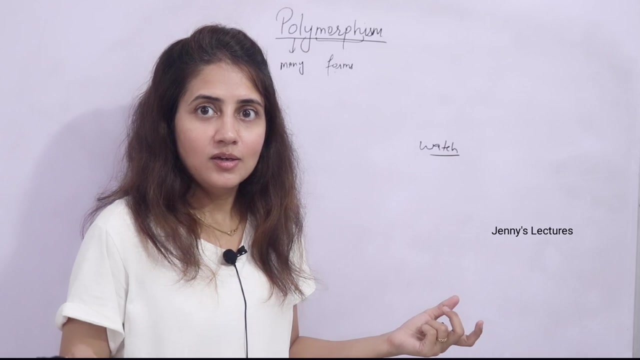 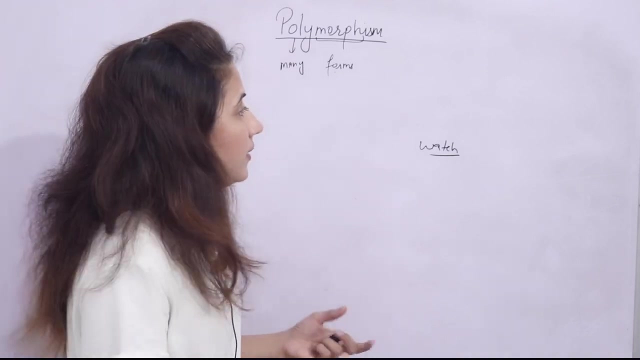 in different way we can use, like you are watching me right now through this video. In this video, Right Watching means dekhna as well as. So this word, same word, but having two different meaning, These kind of we are having many words in English, Right, So this is kind of polymorphic things or polymorphism. Okay. Now in programming, obviously using OOP, object-oriented programming paradigm, we can 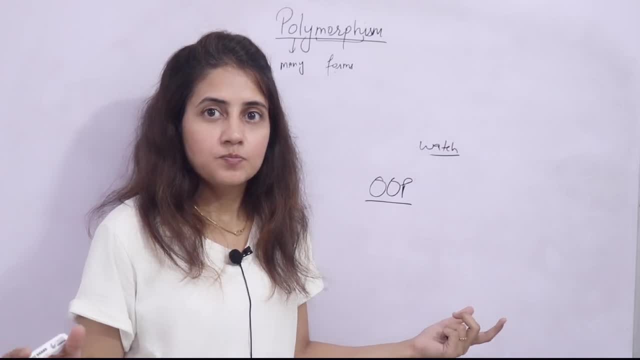 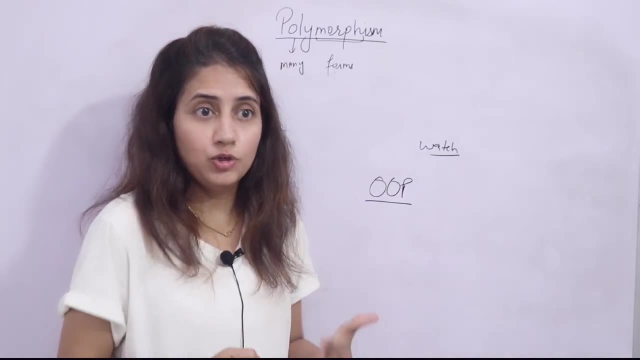 model, the real world objects, right Easy. So that is why, in programming, if you want to, you know, implement this polymorphic behavior, this polymorphism in your program, through your program, and how we are going to achieve this behavior, How we are going to implement this thing, And what is polymorphism in that case? Okay, 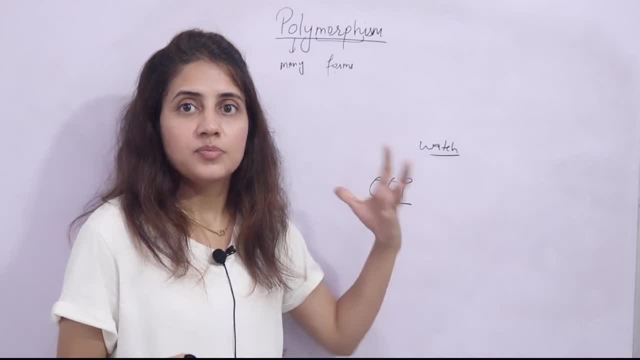 So we can achieve, we can implement polymorphism with. I guess you can four ways here. First is ducktyping, So we can do what, or to dig, occurred, exists, OOP and to find. okay, then we are, You can tell me. 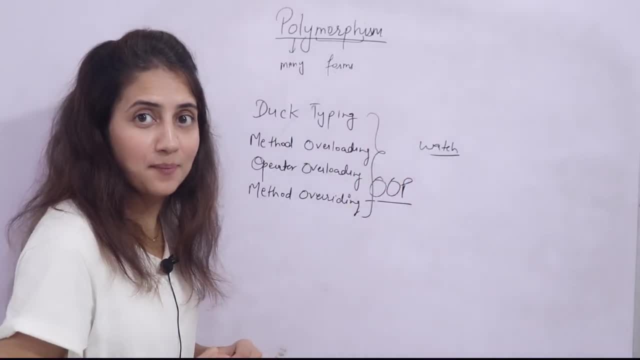 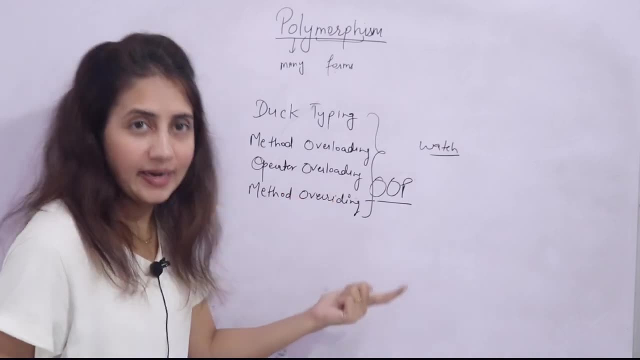 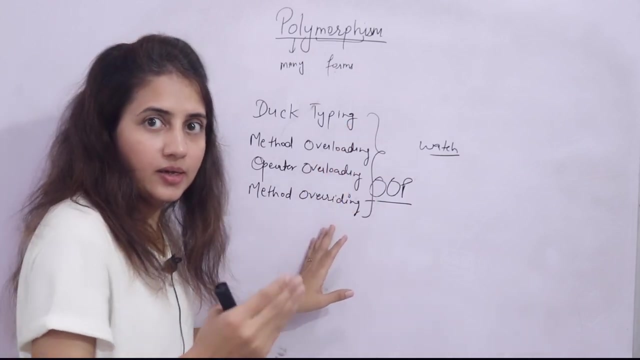 Yeah For the sew. So these are four ways to implement polymorphism in programming, like duct typing, method overloading, operator overloading and method overriding. So what are these techniques and how we are going to achieve this thing with these things that we will see one by one. 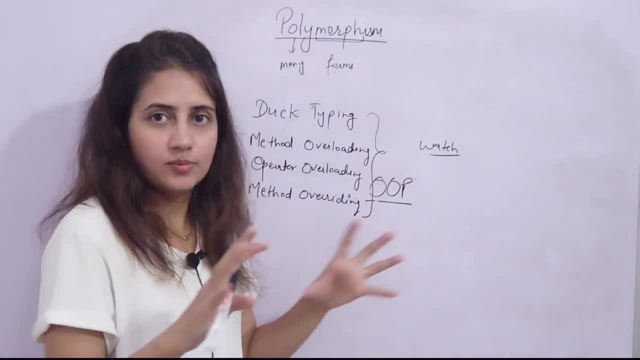 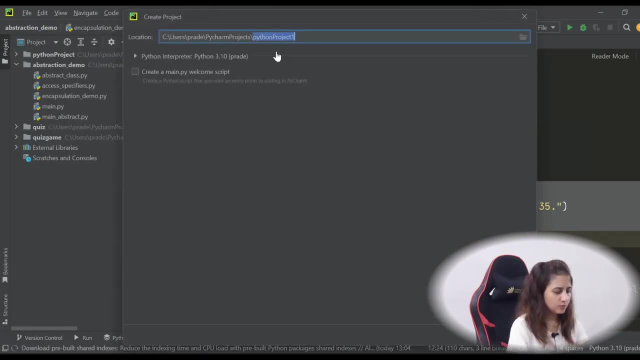 Now let me just show you some practical of this polymorphic behavior or polymorphism. Okay, so let's create a new project here and I am naming this project polymorphism underscore demo. Okay, I am just going to create and I am going to attach this. 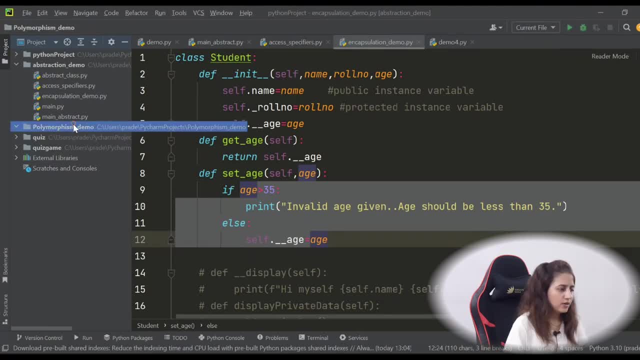 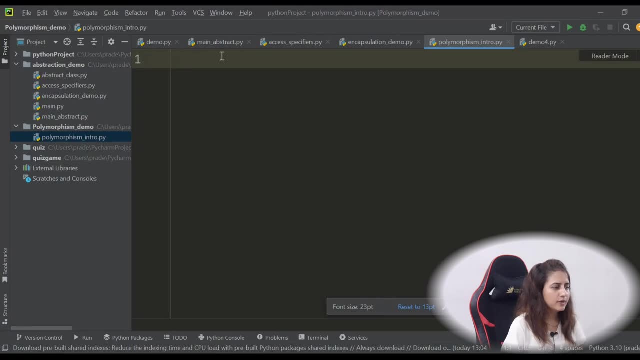 So this is, we got the polymorphic demo. polymorphism demo. Now let's create a new file in this project and polymorphism intro dot py. Okay, Let me just show you the simplest or the basic example of polymorphism: Polymorphism, or having multiple forms. 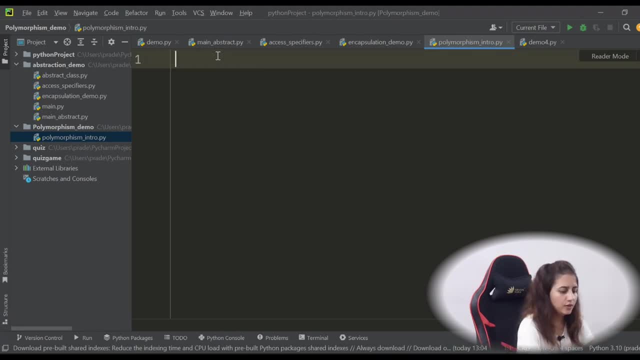 You have plus operator. What it will do? Simply, you will do addition. So if you think, sorry, if you print like print one plus two, what do you think What output you will get? That's very simple: You will get three. 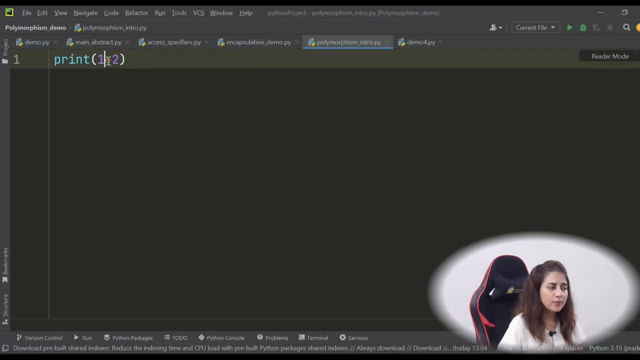 See, you will get three. But if same operator plus- and I am using this operator with one and two- are integer with string, Suppose I am writing one, something like this, plus two, something like this: Now, these are in double quotes, or you can use single quotes as well. 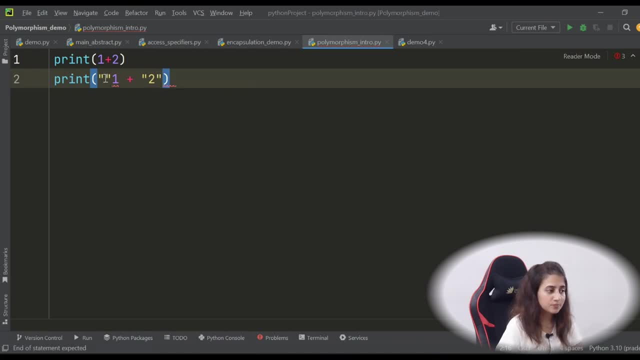 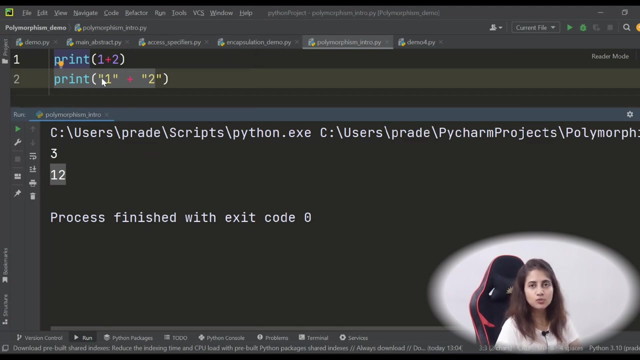 Means these are strings now. Okay, So it would be within these quotes. Now what output you will get for this line. Let's run this: See: for first line it's three, For second line it's one. two means on integer it will work as addition and on string it. 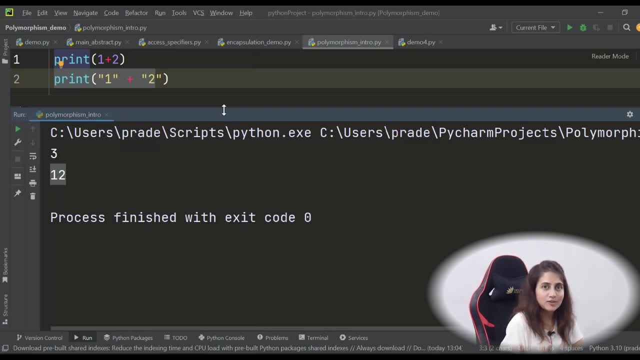 will work as concatenation operator. concatenation, So it's going to concatenate these two strings. So see this: even the operator is same, symbol is same, but having different output in these two lines, having multiple forms, or you can, this is what inbuilt operator. 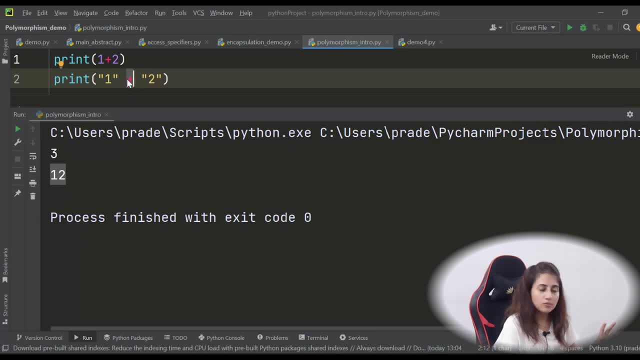 So it's kind of operator overloading. you can say: or you can define your own also, like what this plus will do. You can define that thing at your own. but how you will do that thing I'll show in operator overloading Okay. 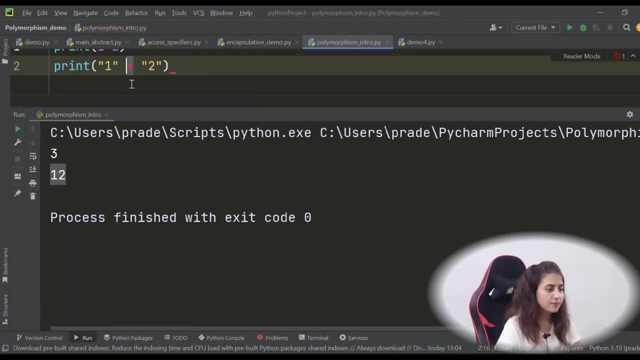 Maybe the operator or the symbol is plus, and you can define your own thing here, the process, and it will do subtract. actually it will do minus, but it will do something else. It will do addition of maybe two objects- You have created two classes, two objects- and addition of those objects, something different. 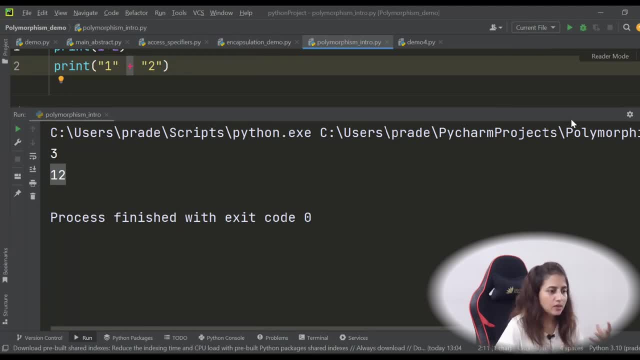 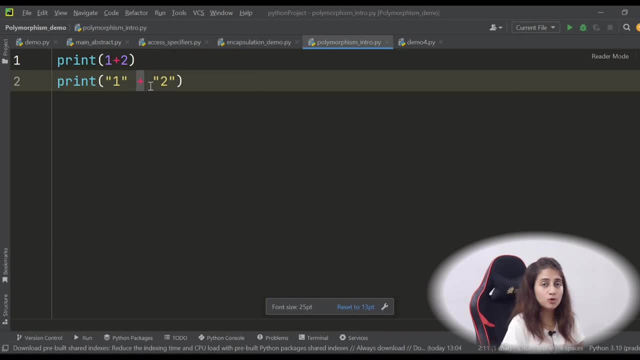 So that behavior you can define yourself. that is operator overloading Right, But that we'll see later. So this is how You can say that this plus is having polymorphism behavior, polymorphic behavior or this is polymorphism Right. So what thing you are going to pass to this plus? because plus is an operator, then operand. 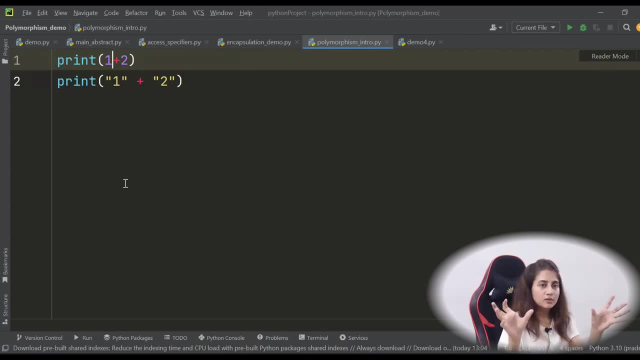 one, operand two. So what operand you are going to pass. the behavior of this plus depends on those operands what you're passing, whether it's a string, whether it's float, whether it's integer- Okay, Same. So let's say example of a function: you have many inbuilt functions. 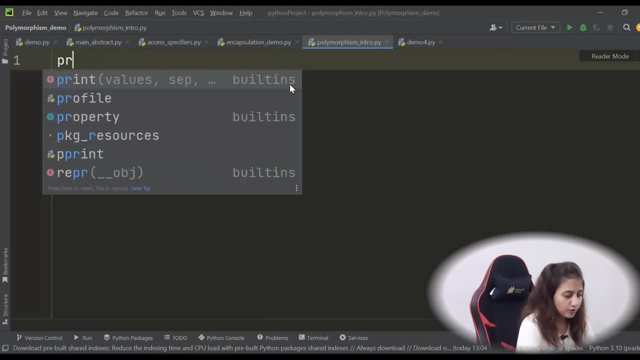 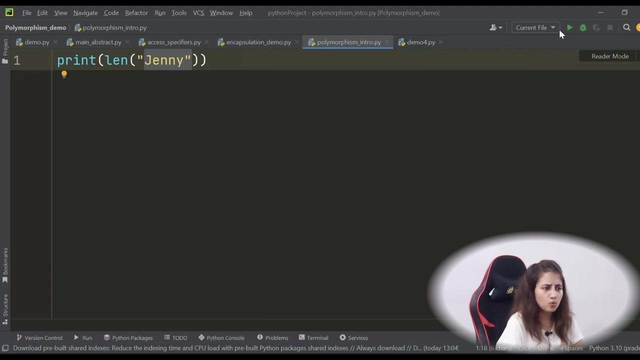 Suppose you have a function, you know we have a function length. So if I use this length function, something like this, I'm using this on Jenny, like Jenny's a string length Jenny. So what it will do, it will print the length of the string. 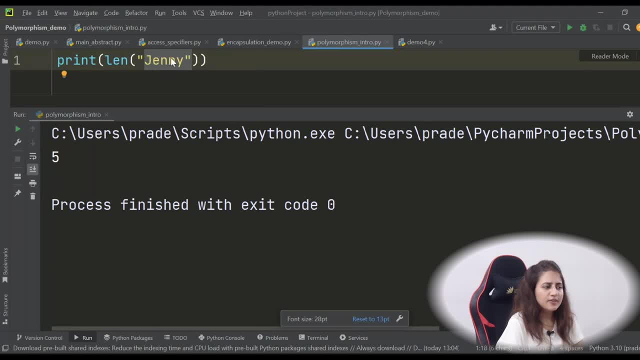 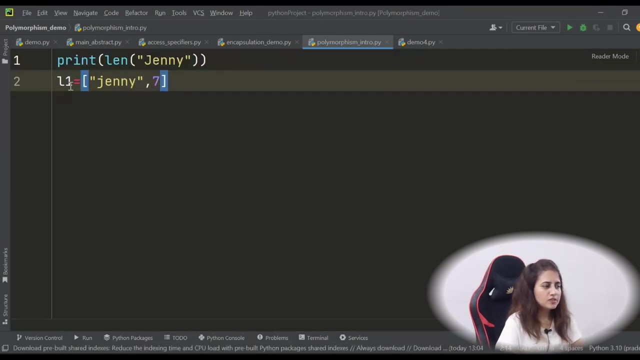 So what should be the output? that is five means it is going to count the number of characters, Right, Okay, So if I have a list, suppose I have a list L1, and in this list I have one item as Jenny. second is seven. 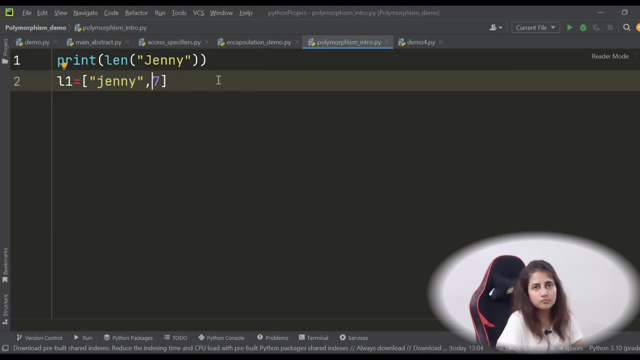 This is a list, Jenny, seven or anything you can have, because list we can have multiple mix of mixed data type: string, int, maybe boolean or something else, Right, And if I print now, I've applied this length function on this list L1.. See what is going to happen. 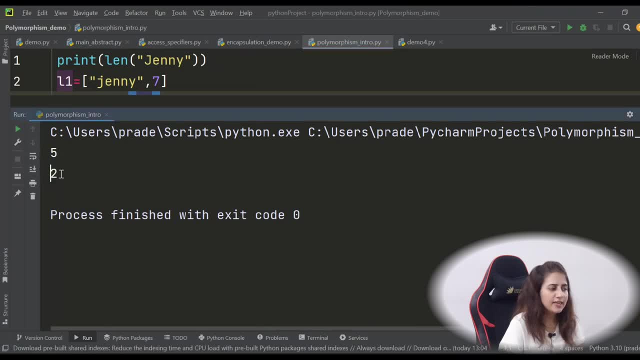 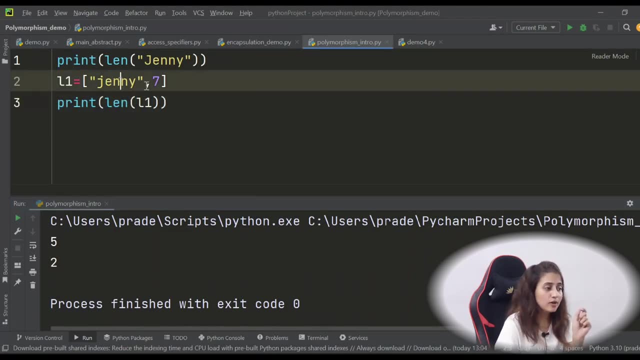 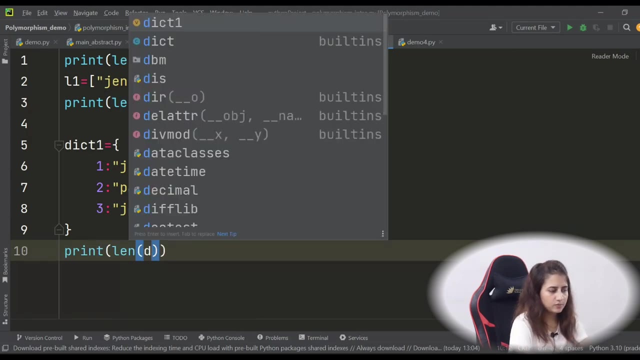 Now the output of first line is five. output of second line is two. For this line it is going to print. two means it is going to print number of item in the list: one, two. Okay, So I have this dictionary and I'm going to apply this length function on this dictionary. 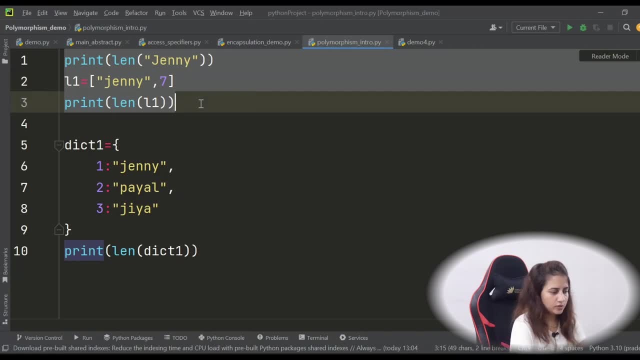 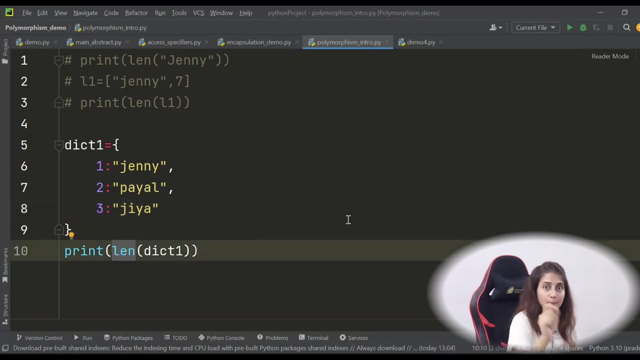 to one. Let's just comment out these lines. So what it is going to print now, this length function, See, the output is three. It is going to count the number of key value pair One, two and three. So this length function, the name is same function, name is same length, but the output and the